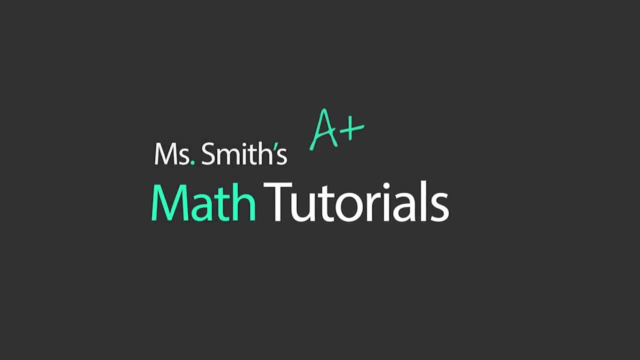 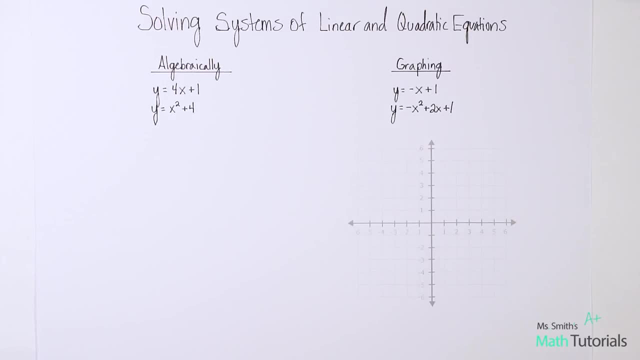 Welcome to Ms Smith's Math Tutorials. I'm Ms Smith. In this video, we're going to be talking about solving systems of linear and quadratic equations. Now we're both going to do this algebraically and graphically, And then, after we do it through graphing, I'm going to show you how. 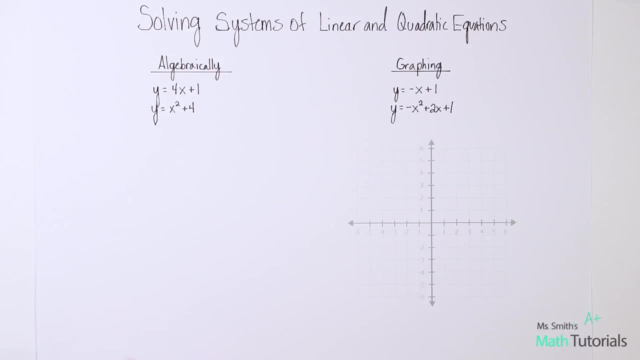 you can also do it on your calculator, So let's dive right in. So remember, a system is two equations. One will be linear. So in this example, this first one's our linear equation. Remember, linear equations are to the power of one. Your highest exponent on a variable would be one. 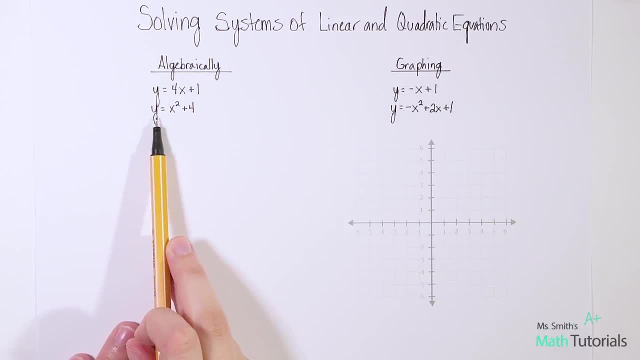 And then a quadratic equation, which in this case would be our second equation. So its highest power on a variable is two. What I want you to recognize that this is y equals 4x plus one, and this is y equals x squared plus four. 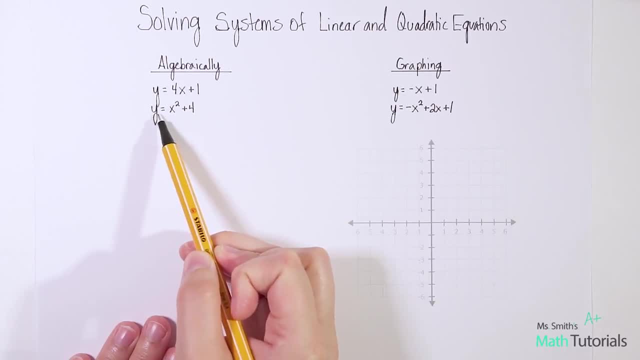 So if y equals this and y also equals this, then these two things equal each other. So that's an equation that we can write. So we can write: 4x plus one equals x squared plus four. If this equals this and this equals this, then this equals this. Now, at this point, I want to get: 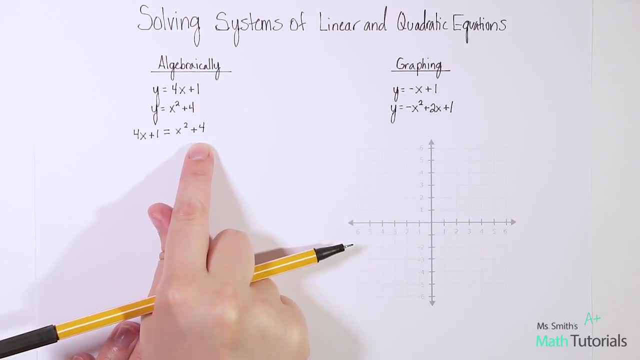 everything together on one side of the equation. So I'm going to do this. So I'm going to do this equation. A lot of students are tempted to say, okay, well, let's subtract x squared and move it over here. Technically you can do that. I don't recommend it. I always recommend keeping the x. 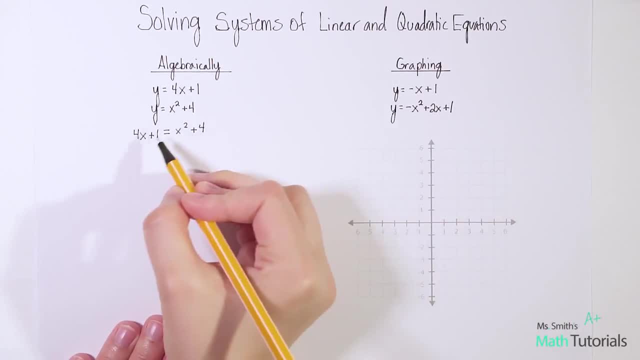 square positive, just to keep things clean and simple. All right, so move the 4x by subtracting it over here. Whatever is the x squared side, you want to go to that side. Now let's see. So we've got this point. just a one equals x squared. I know like terms here I can combine, So it would. 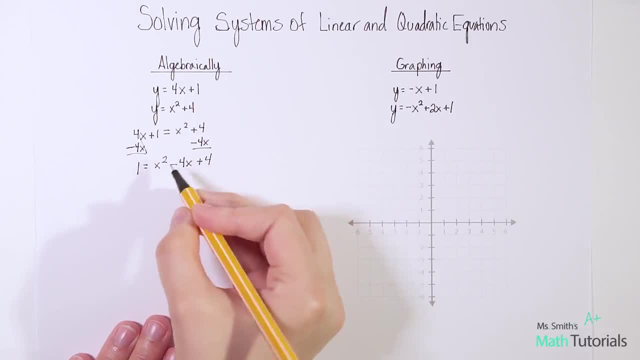 just be negative: 4x plus four. We always want to write our answer in standard form. Okay, constant last. Of course, I don't want this to be equal one, I want it to be equal zero. So now I need to subtract one from each side, So I've got zero equals x squared minus four x four. 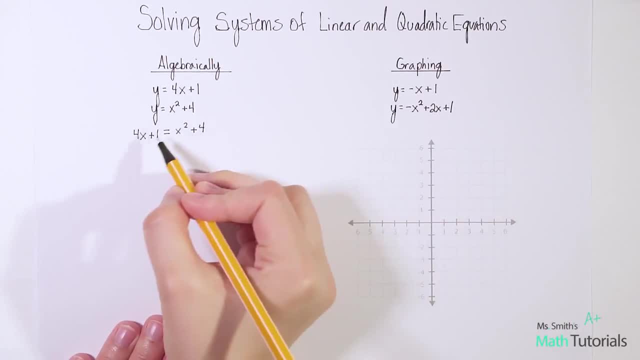 square positive, just to keep things clean and simple. All right, so move the 4x by subtracting it over here. Whatever is the x squared side, you want to go to that side. Now let's see. So we've got this point. just a one equals x squared. I know like terms here I can combine, So it would. 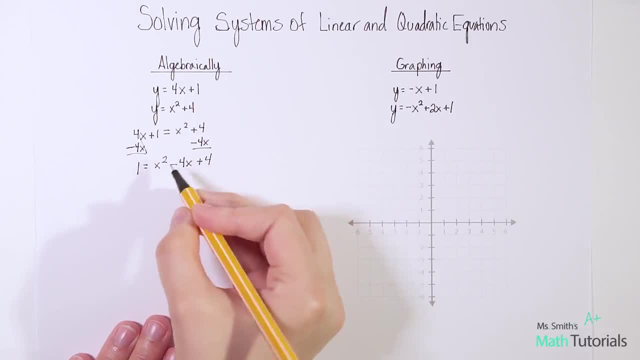 just be negative: 4x plus four. We always want to write our answer in standard form. Okay, constant last. Of course, I don't want this to be equal one, I want it to be equal zero. So now I need to subtract one from each side, So I've got zero equals x squared minus four x four. 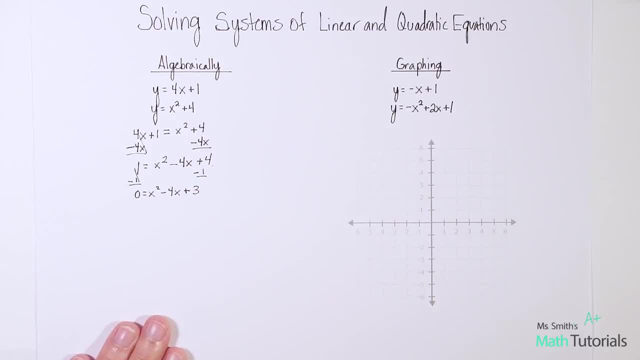 minus one is positive three. So now I've got this all combined together into one quadratic equation that I can solve. Okay, so let's go ahead and label my A, which would be one, my B, which would be negative four, and my C, which would be three. Now, if you're not sure what I'm talking about, 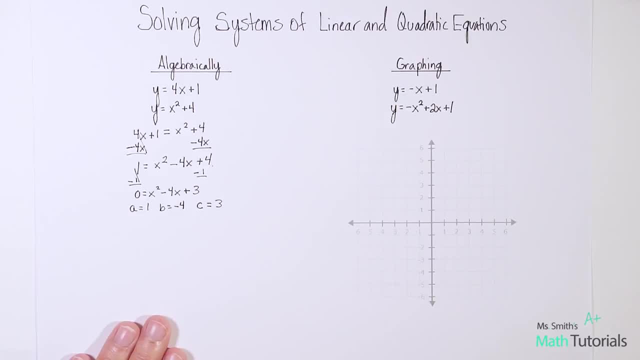 when I say quadratic formula, you definitely want to stop and go watch my video on the using the quadratic formula. before you watch this video, Remembering my quadratic formula, remember that it is negative, B, negative, negative, four plus or minus square root of B, So negative. 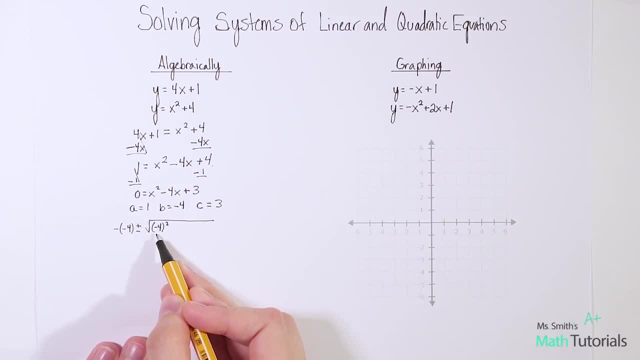 four squared. You must have parentheses around that negative four. If you do not, your answer will be wrong. Okay, so, negative four squared B squared minus four times A times C, all over two times A. Remember, when we use the quadratic formula, we first simplify what. 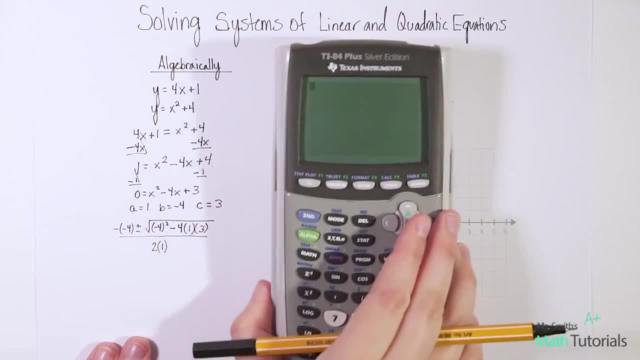 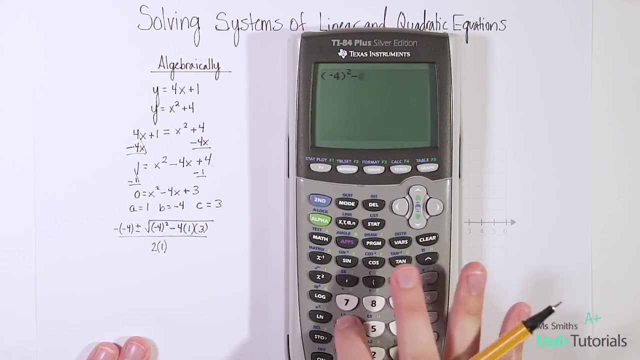 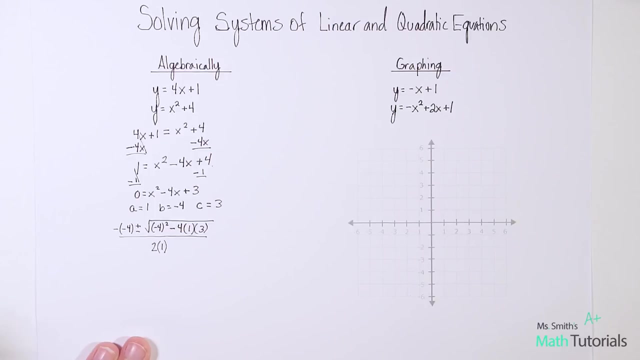 we have underneath the radical. So let's use our calculator to do that, Save some time. Negative four squared must have those parentheses minus four times one times three. All right, and we get four. So that means we've got negative four squared minus four times one times three. 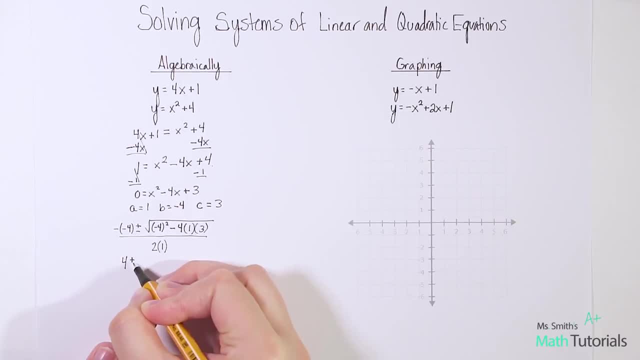 And that's the negative square root of everything that's going down. Okay, now we'll see more of that in a second. So that is negative plus or minus square root of everything that's going down. Negative times, the negative, remember that's a positive four plus or minus the. 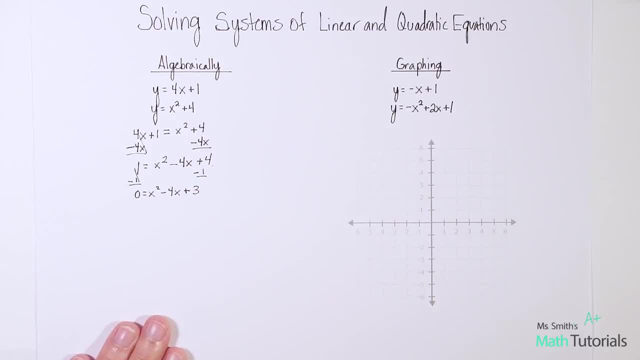 minus one is positive three. So now I've got this all combined together into one quadratic equation that I can solve. Okay, so let's go ahead and label my A, which would be one, my B, which would be negative four, and my C, which would be three. Now, if you're not sure what I'm talking about, 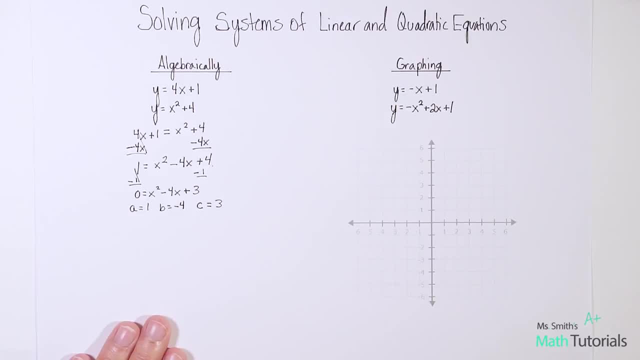 when I say quadratic formula, you definitely want to stop and go watch my video on the using the quadratic formula. before you watch this video, Remembering my quadratic formula, remember that it is negative, B, negative, negative, four plus or minus square root of B, So negative. 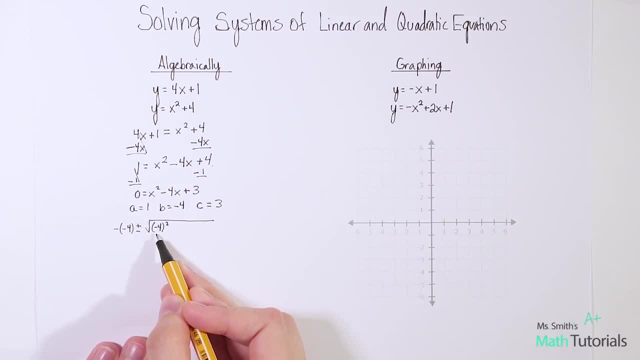 four squared. You must have parentheses around that negative four. If you do not, your answer will be wrong. Okay, so, negative four squared B squared minus four times A times C, all over two times A. Remember, when we use the quadratic formula, we first simplify what. 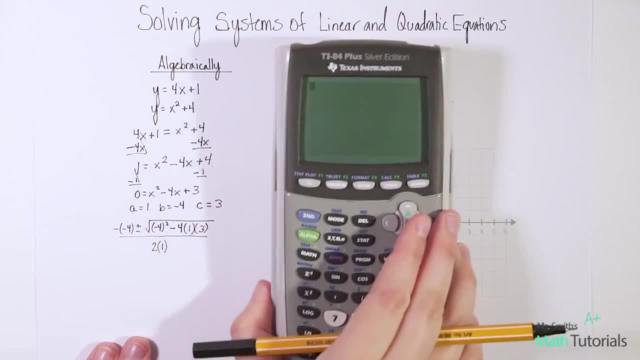 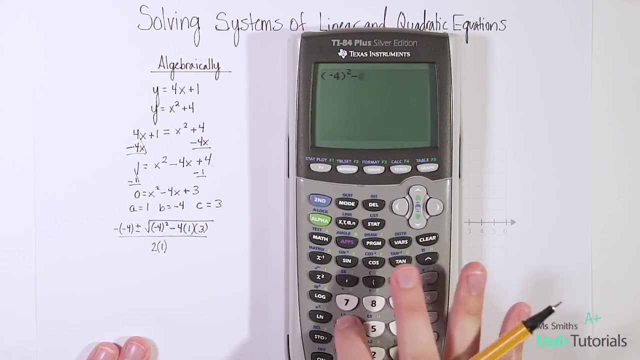 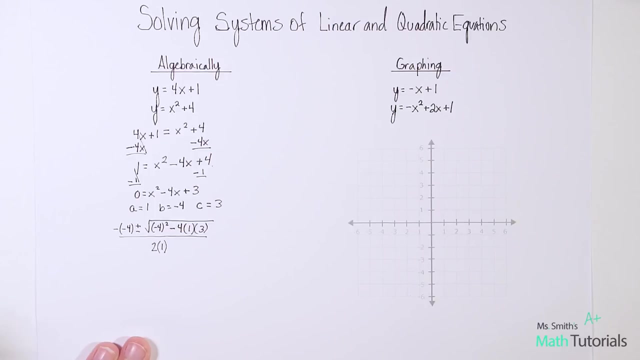 we have underneath the radical. So let's use our calculator to do that, Save some time. Negative four squared must have those parentheses minus four times one times three. All right, and we get four. So that means we've got negative four squared minus four times one times three. 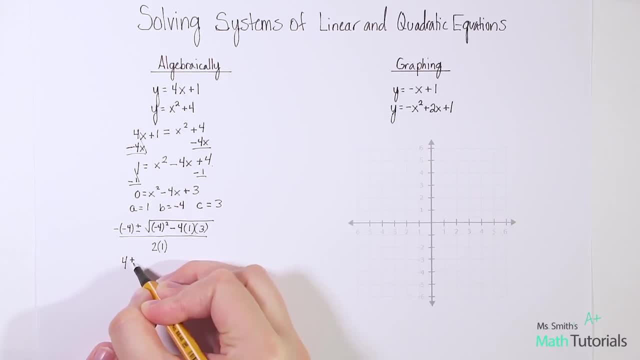 Quadrate plus or minus the square root of four all over two times 1, that becomes negative. Y over X, minus negative Times, a negative, Remember. that's a positive. four plus or minus the square root of four all over 2 times one is 2.. OK, So can we. 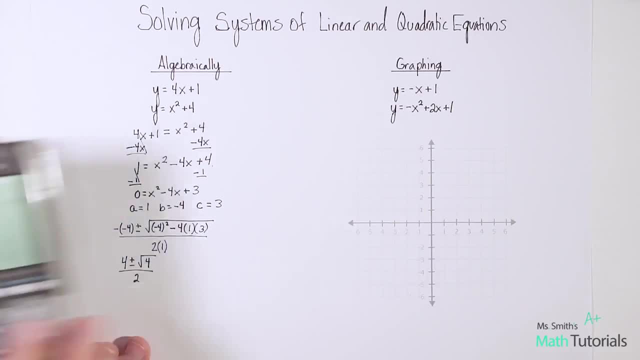 Can we simplify square root of four? Does that reduce? Is that a perfect square? Let's check Square root of four and we get two. We get a nice whole number. So that reduces really well to four plus or minus two, all over two. 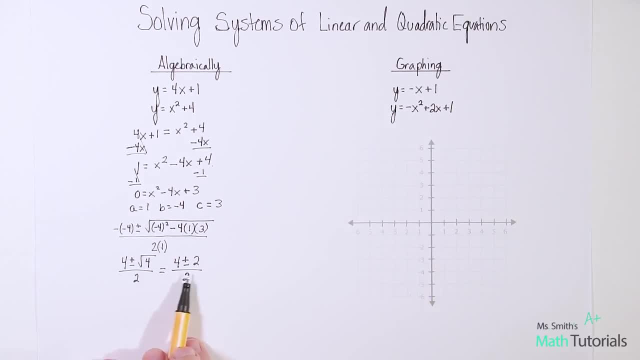 So that reduces really well to four plus or minus two, all over two. Yay, So this is technically two separate statements written in one. We have our 4 plus 2 over 2. That covers that positive. And then we also have our 4 minus 2 over 2.. 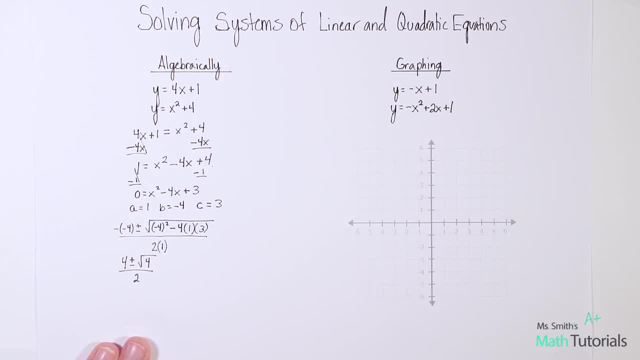 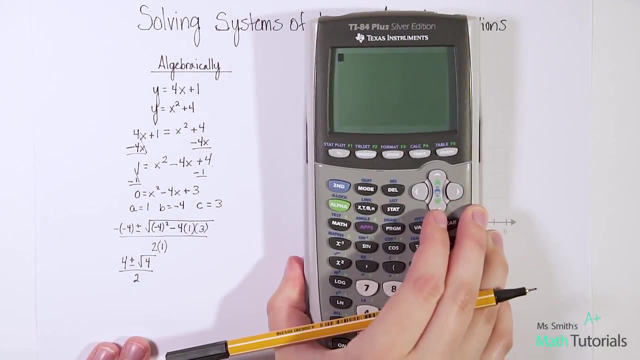 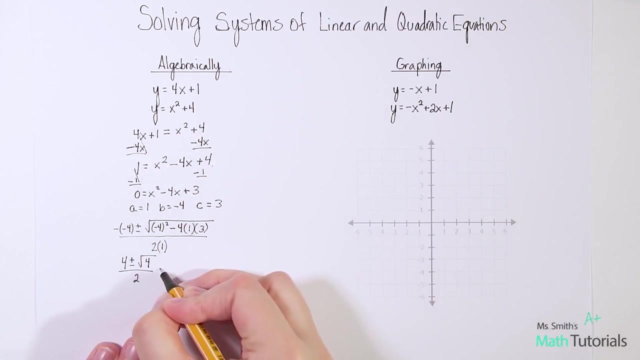 square root of four all over two times one is two. Okay, so can we simplify square root of four? Okay, does that reduce? is that a perfect square? Let's check Square root of four and we get two. We get a nice whole number. So that reduces really well to four. 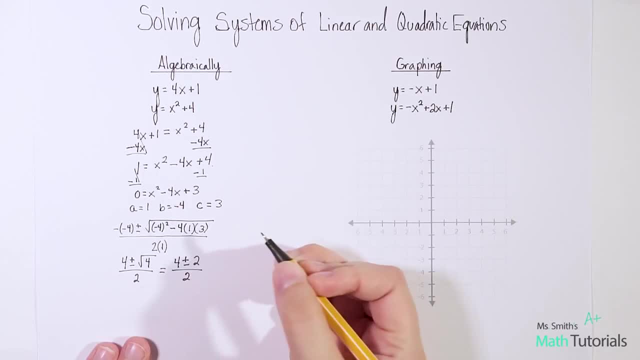 plus or minus two, all over two Subtitles by the Amaraorg community. So this is technically two separate statements written in one. We have our 4 plus 2 over 2. That covers that positive. And then we also have our 4 minus 2 over 2.. 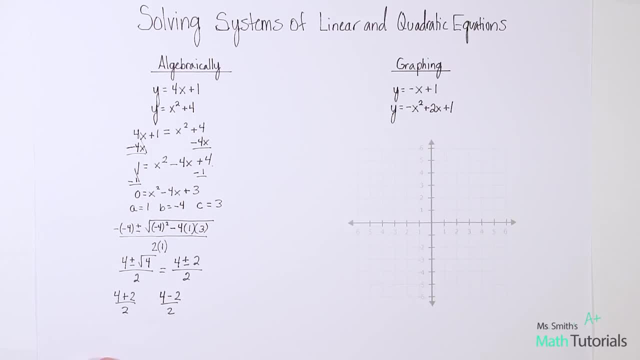 Okay, so let's solve both of these and figure out what is x. So 4 plus 2 is 6.. 6 divided by 2 is 3.. And then we have 4 minus 2, which is 2.. 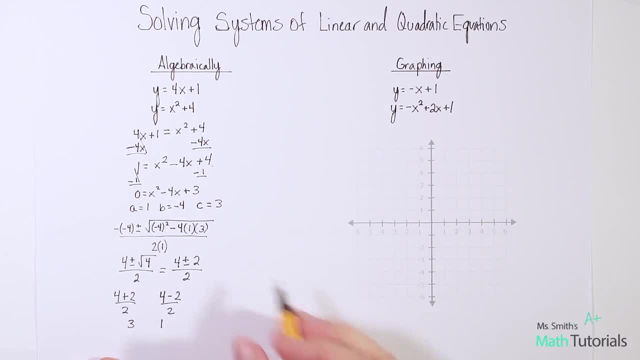 2 divided by 2, which is 1.. So we know that our solutions here is x is the could be 1 and 3.. Okay, So here's the thing, though We're not quite done, Because it's great to know that x is 1 and 3, but I want to know the system. 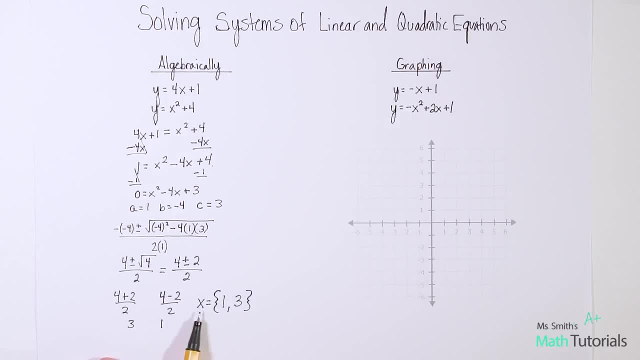 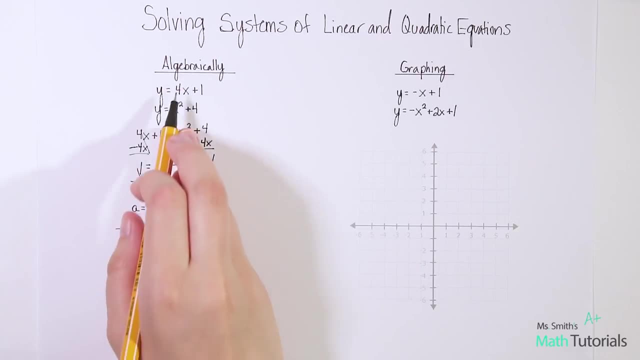 I want to know the actual intersecting points, right, I don't want to know. 2. I want to know just the x values. I want to know the y values as well. So we're going to want to take each of these x values back up to an original equation and 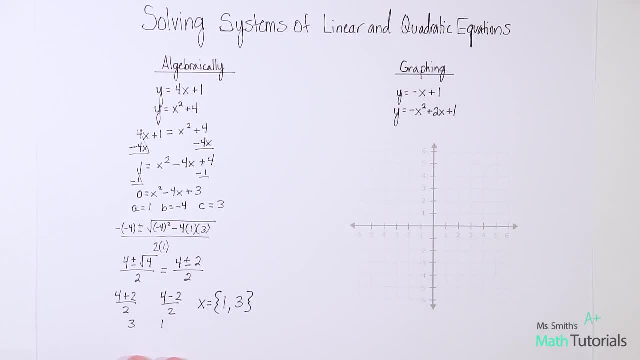 figure out what will be my corresponding y values. Okay, I can pick either equation. I would pick the top one, just because I don't want to deal with a square, I'd rather just deal with a linear equation. So, one at a time, I'm going to plug in each of these x values. 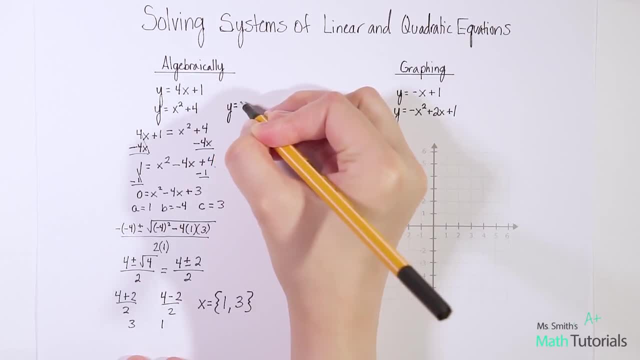 So first we'll do y equals- Okay, Y equals 4 times x. But first we're going to do 1.. 4 times 1 plus 1. 4 times 1 is 4, plus 1 is 5.. 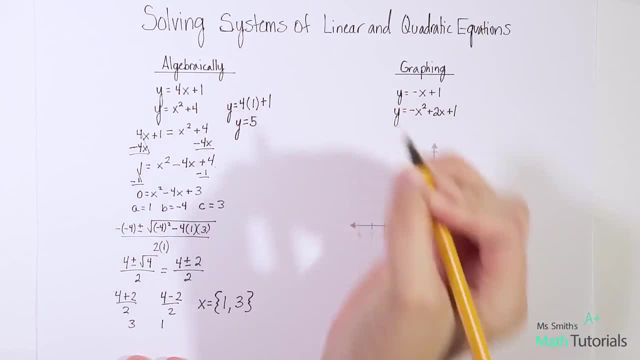 So I know that one of my solutions is 1 comma 5.. I'm going to write my official answer- just I don't know- right down here. So my final answer, One intersecting point, would be at 1 comma 5.. 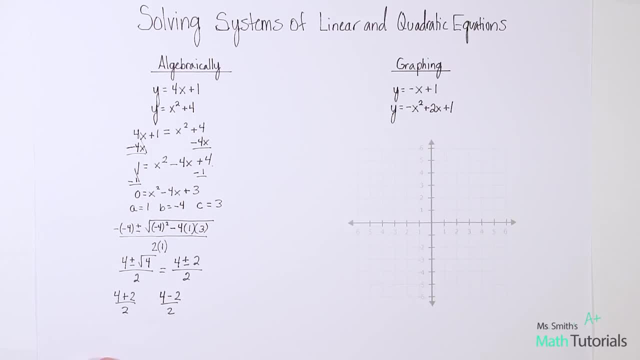 Okay, so let's solve both of these and figure out what is x. So 4 plus 2 is 6.. 6 divided by 2 is 3.. And then we have 4 minus 2, which is 2.. 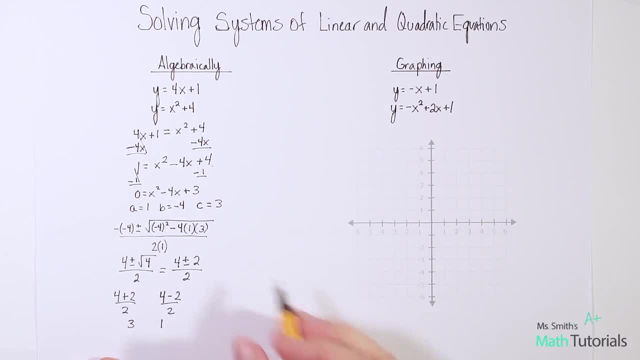 2 divided by 2, which is 1.. So we know that our solutions here is x is the could be 1 and 3.. Okay, So here's the thing, though We're not quite done, Because it's great to know that x is 1 and 3, but I want to know the system. 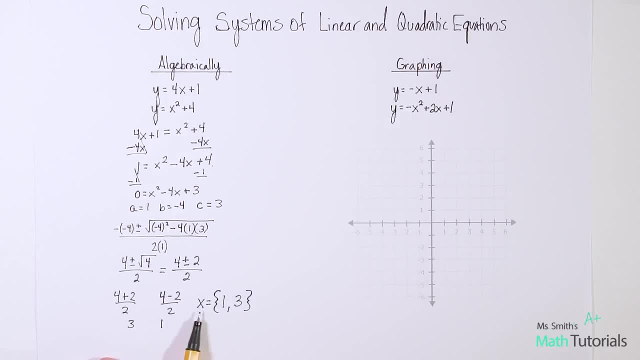 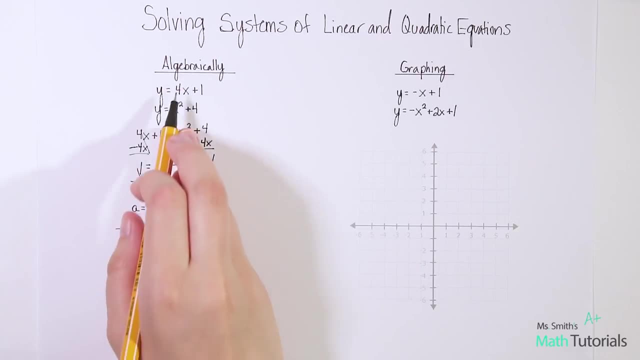 I want to know the actual intersecting points, right, I don't want to know. 2. I want to know just the x values. I want to know the y values as well. So we're going to want to take each of these x values back up to an original equation and 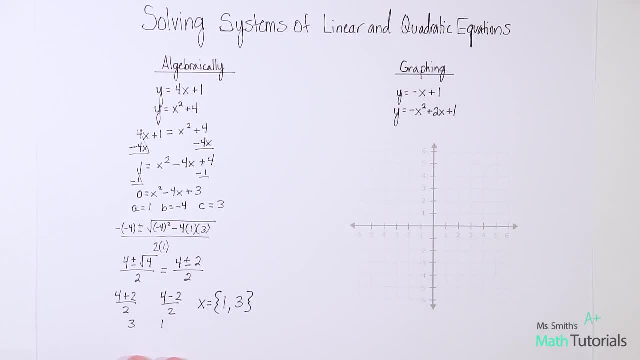 figure out what will be my corresponding y values. Okay, I can pick either equation. I would pick the top one, just because I don't want to deal with a square, I'd rather just deal with a linear equation. So, one at a time, I'm going to plug in each of these x values. 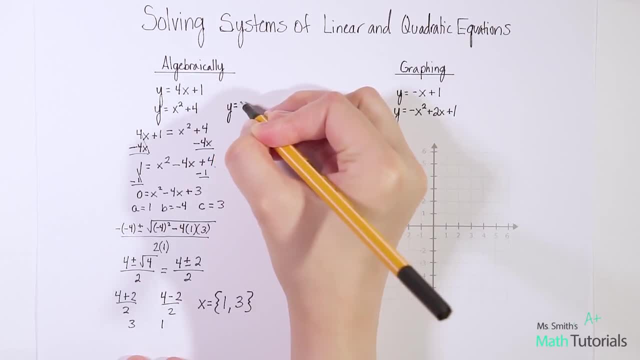 So first we'll do y equals- Okay, Y equals 4 times x. But first we're going to do 1.. 4 times 1 plus 1. 4 times 1 is 4, plus 1 is 5.. 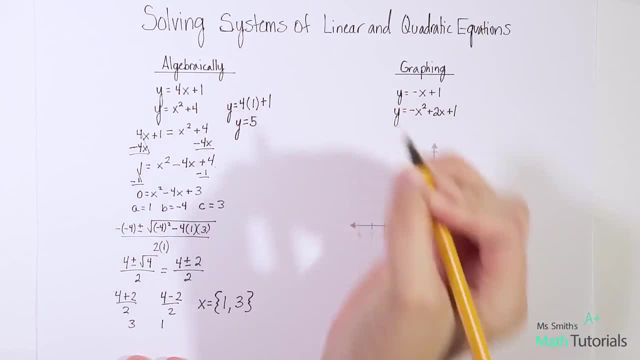 So I know that one of my solutions is 1 comma 5.. I'm going to write my official answer- just I don't know- right down here. So my final answer, One intersecting point, would be at 1 comma 5.. 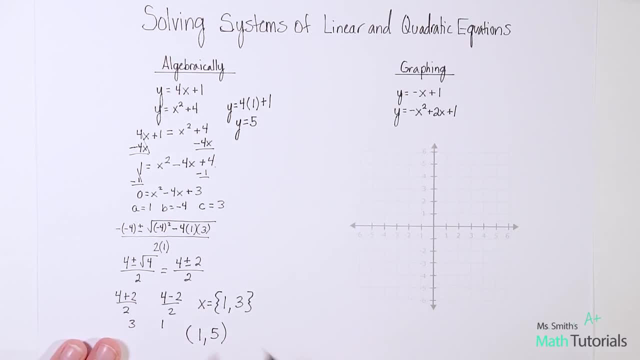 And the other intersecting point. I know the first, the x would be 3, but let's figure out what the y would be. So I would go back to the same equation: Y equals 4 times 3 plus 1.. 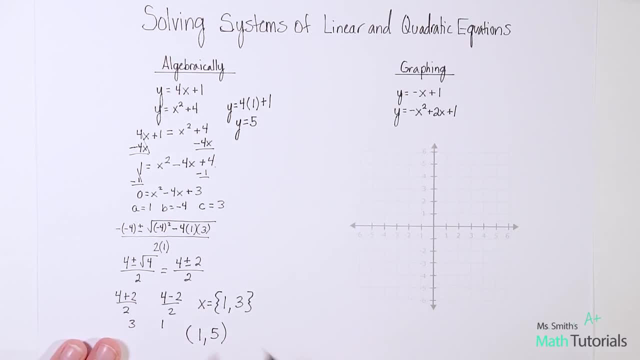 And the other intersecting point. I know the first, the x would be 3, but let's figure out what the y would be. So I would go back to the same equation: Y equals 4 times 3 plus 1.. 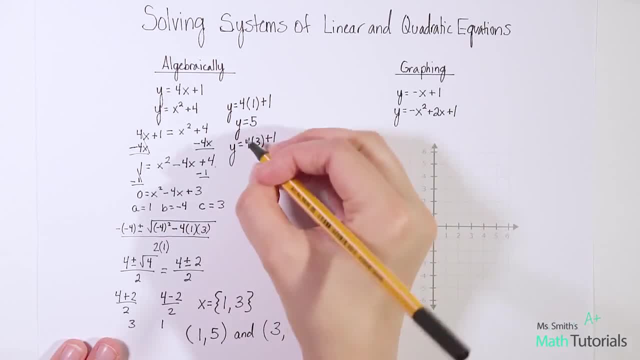 4 times 3 is 12. And 12 plus 1 is 13.. 3 comma 13.. So those are my two intersecting points. What are my two intersecting points? That is most definitely the long way around. 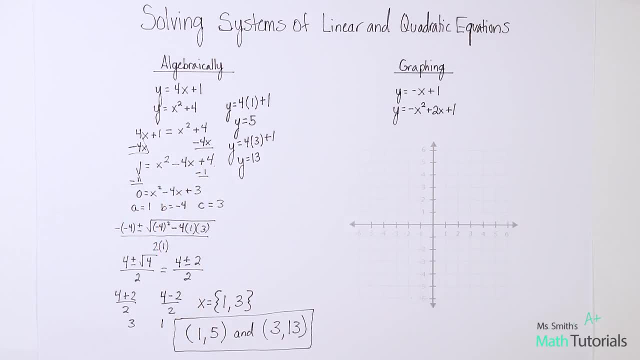 Solving algebraically is a longer method to get your answer, but it's something you do need to know how to do And the reason why you need to know. some people might say: well, I'm always going to have a calculator with me. 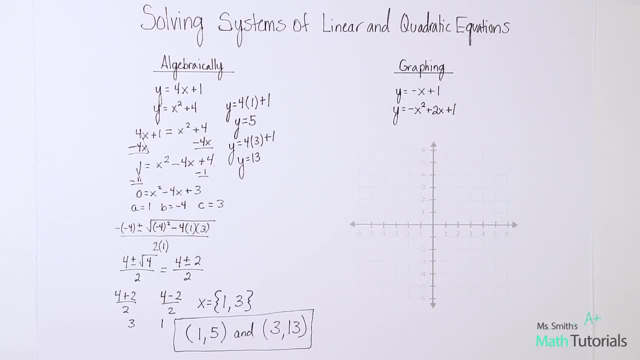 Well, what if you get in a test so at some point in your math career and it's calculator inactive and they ask you to solve system of linear and quadratic equations? You've got to know how to do it by hand as well. I would never use this unless I have to. 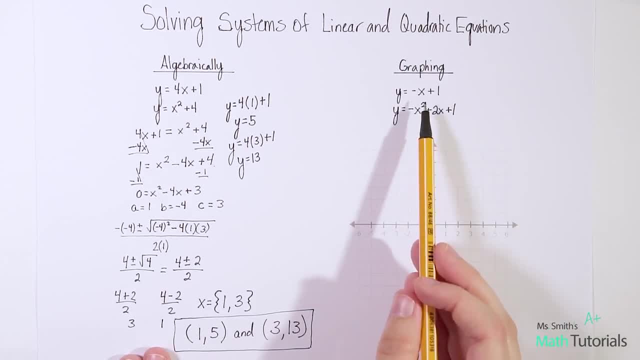 It's good to know how to do it. Let's get to the shorter methods In terms of manually graphing this, which we could do, okay, and I'm going to show you an even shorter way in a minute- but let's go ahead and use our graphing calculator to 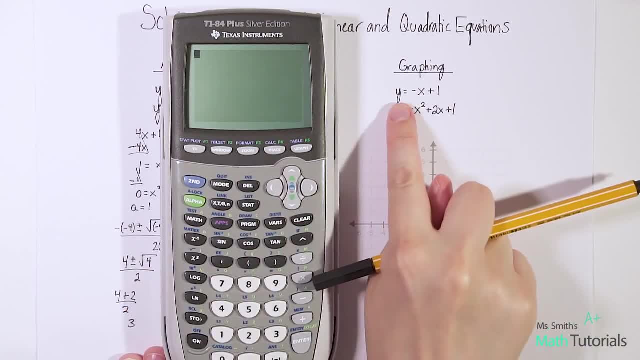 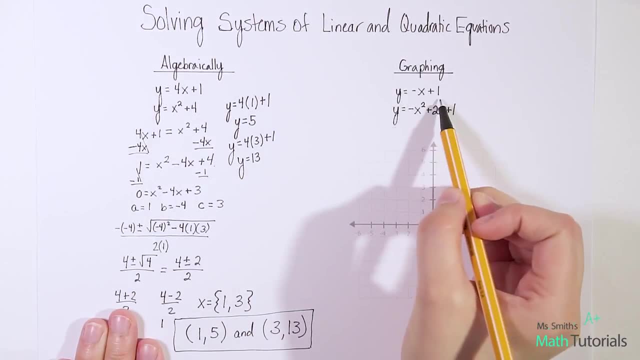 help us. First I need to graph this first line and then I will graph the second line. Now the first line. I actually I don't even need the calculator. I could graph this one by hand, right? It's just a linear equation. 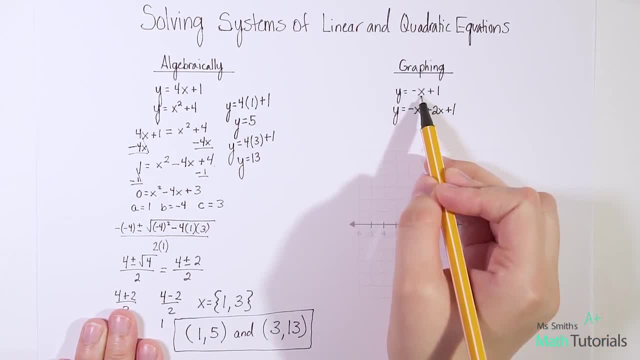 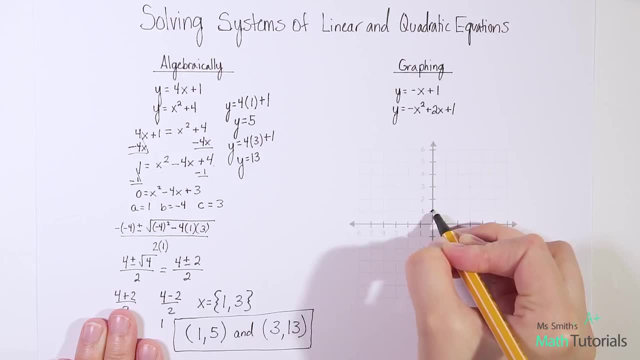 So remember linear equations. this is Y equals MX plus B. Remember B is my starting point. So it starts, my Y intercept starts at positive one And then my slope tells me to move it's negative one. So that means I move down one right one, right down one right one, and I keep this. 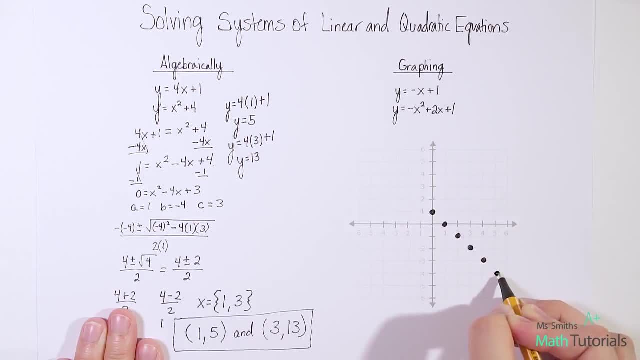 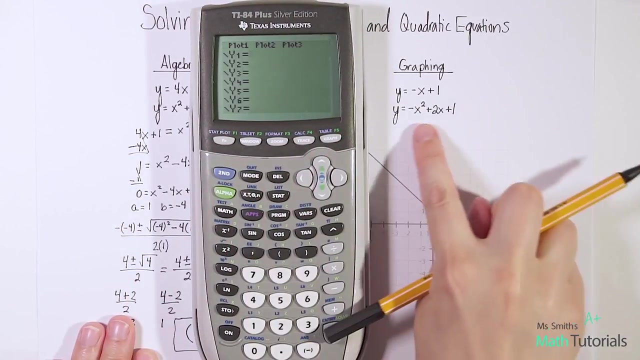 pattern up down one right one. So there's my linear equation. Now for my quadratic equation. I definitely want to bring the calculator in to help me. I would go to my Y equals and type in negative X squared plus two, X plus one. 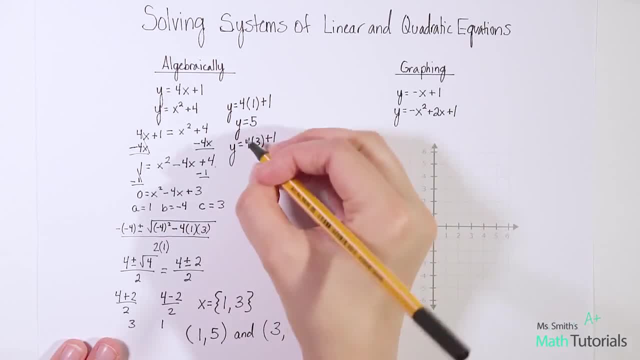 4 times 3 is 12. And 12 plus 1 is 13.. 3 comma 13.. So those are my two intersecting points. What are my two intersecting points? That is most definitely the long way around. 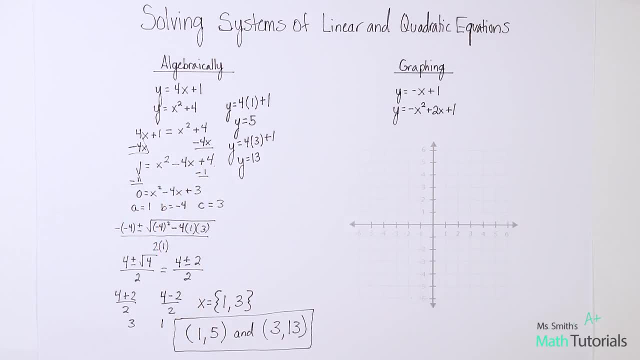 Solving algebraically is a longer method to get your answer, but it's something you do need to know how to do And the reason why you need to know. some people might say: well, I'm always going to have a calculator with me. 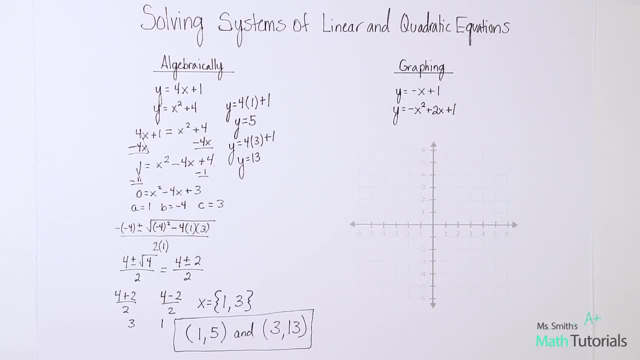 Well, what if you get in a test so at some point in your math career and it's calculator inactive and they ask you to solve system of linear and quadratic equations? You've got to know how to do it by hand as well. I would never use this unless I have to. 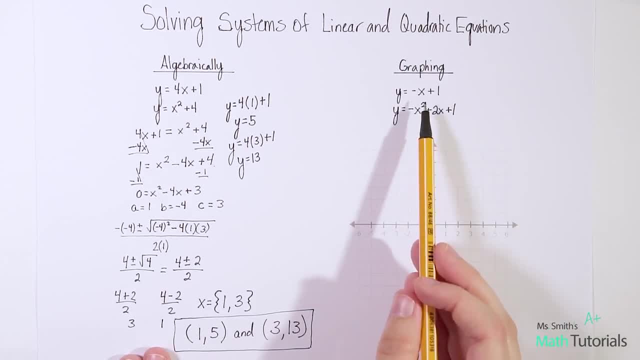 It's good to know how to do it. Let's get to the shorter methods In terms of manually graphing this, which we could do, okay, and I'm going to show you an even shorter way in a minute- but let's go ahead and use our graphing calculator to 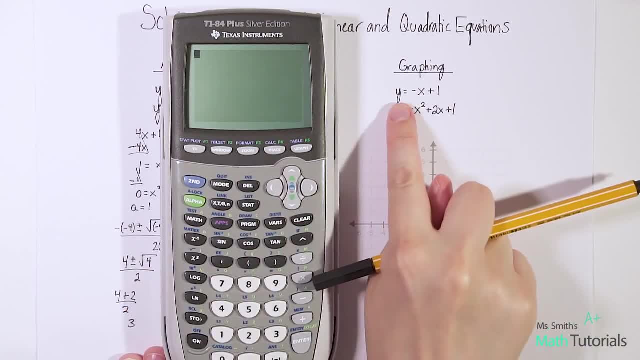 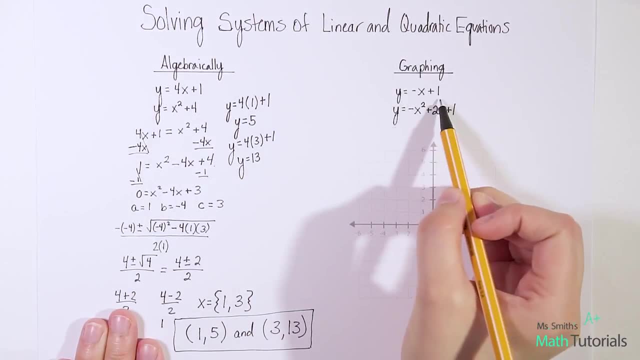 help us. First I need to graph this first line and then I will graph the second line. Now the first line. I actually I don't even need the calculator. I could graph this one by hand, right? It's just a linear equation. 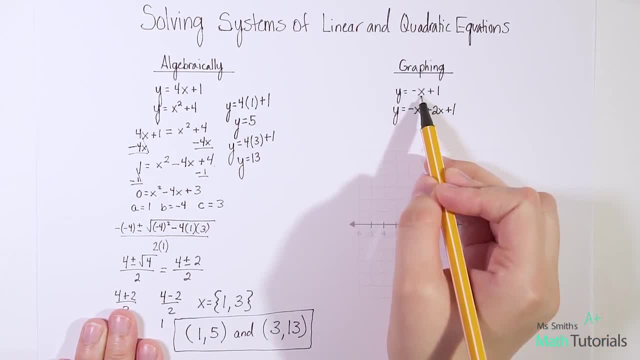 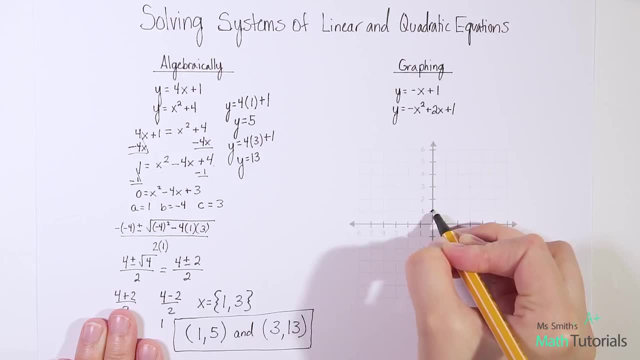 So remember linear equations. this is Y equals MX plus B. Remember B is my starting point. So it starts, my Y intercept starts at positive one And then my slope tells me to move it's negative one. So that means I move down one right one, right down one right one, and I keep this. 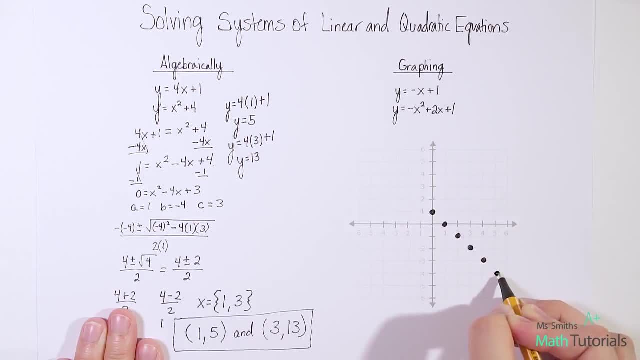 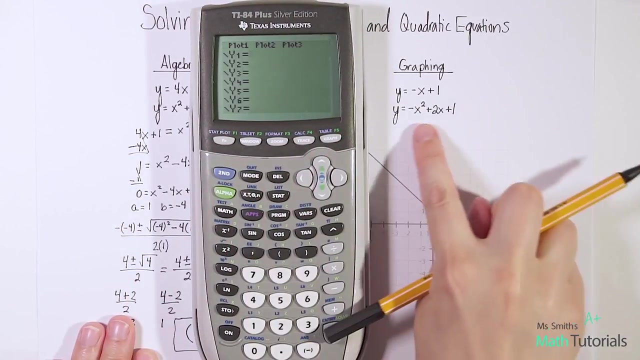 pattern up down one right one. So there's my linear equation. Now for my quadratic equation. I definitely want to bring the calculator in to help me. I would go to my Y equals and type in negative X squared plus two, X plus one. 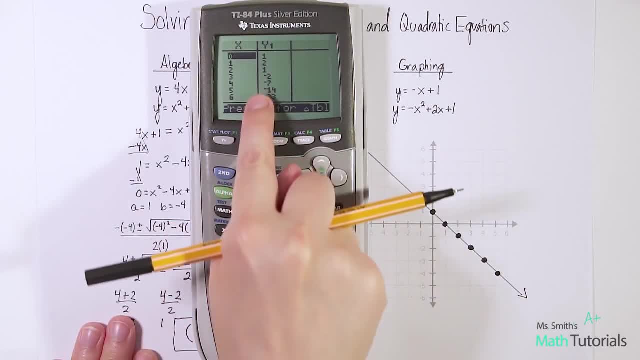 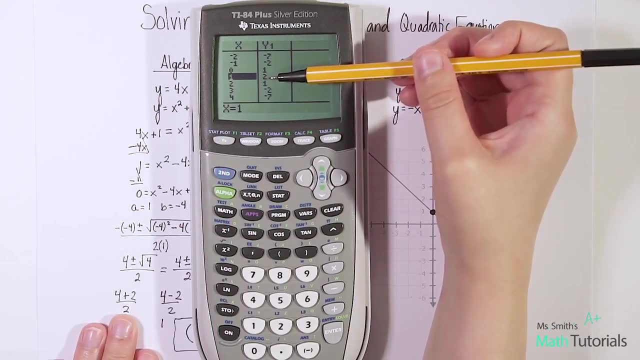 Okay, now let's go to second graph to look at my table of values. Now I want to pick good values. I definitely want to choose the vertex which- remember that's a mirrored image- right? Everything above it and below it is mirrored. 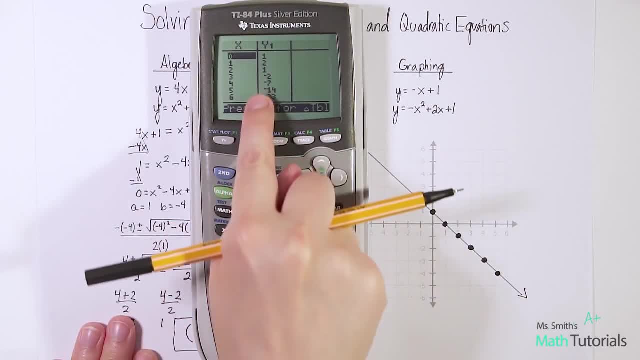 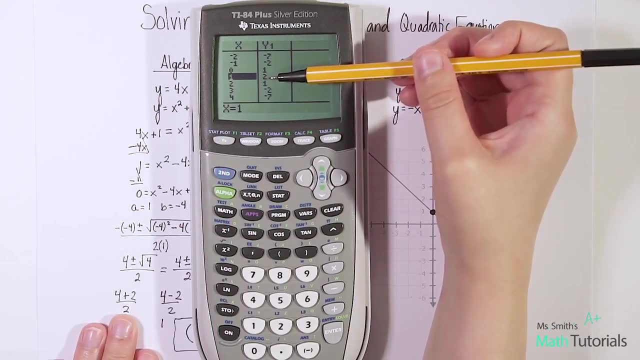 Okay, now let's go to second graph to look at my table of values. Now I want to pick good values. I definitely want to choose the vertex which- remember that's a mirrored image- right? Everything above it and below it is mirrored. 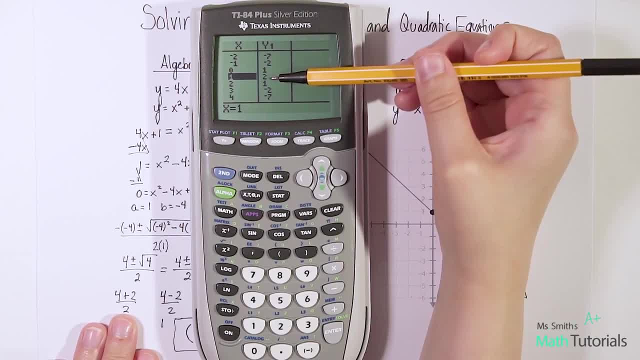 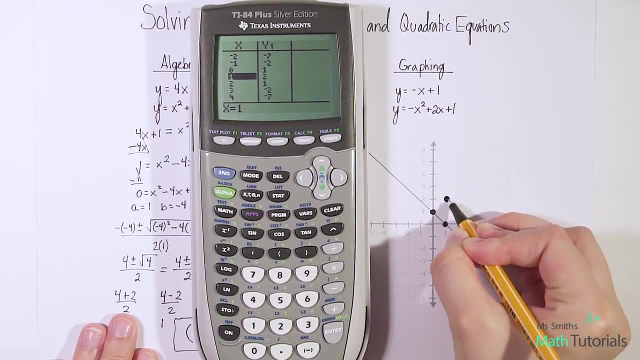 So it creates this kind of cool pattern effect. So you want to definitely have the vertex in there, which falls at one two. let me go ahead and plot that one two and then we'll plot around it. So then I've got zero positive one, zero positive one right there and negative one negative. 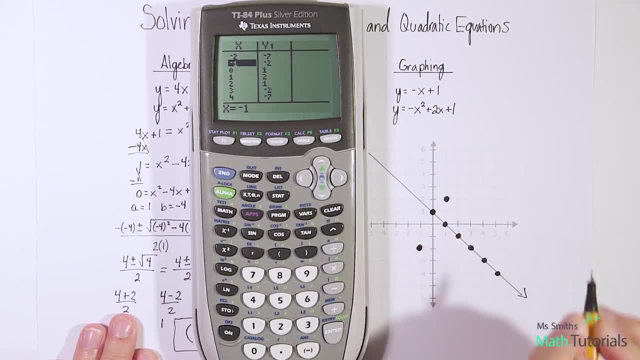 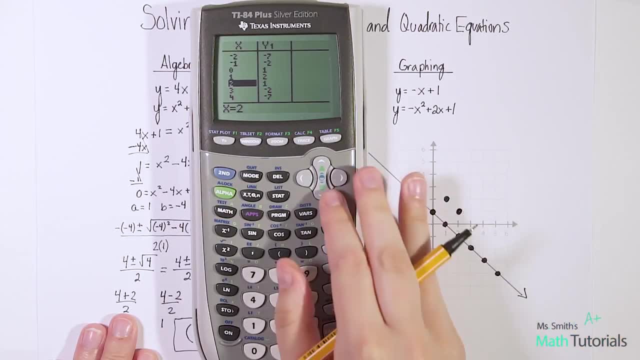 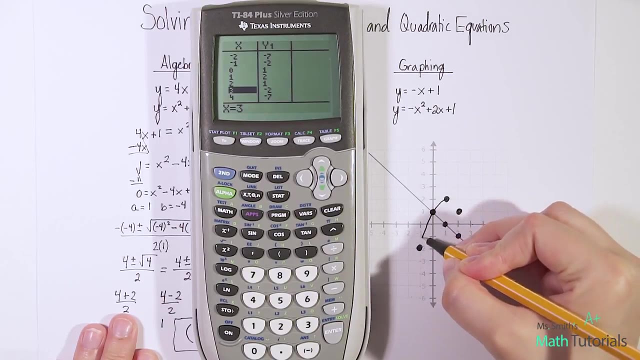 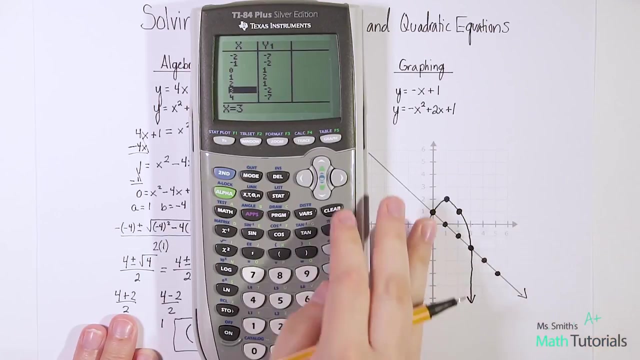 two negative, one negative two. Okay, Okay, Okay. So now I've got a little bit above the vertex. two, one, three negative two, all right, And we'll connect those dots in our parabola form. 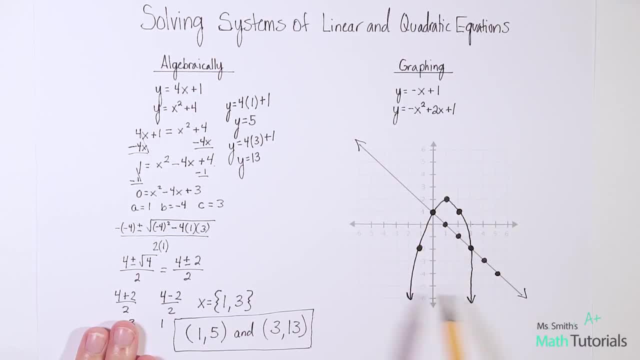 We want to physically see where. I've got my linear equation, I've got my quadratic equation. Where do they intersect? Well, I can. I can clearly see that they intersect right here at zero one and they intersect right here at three negative two. 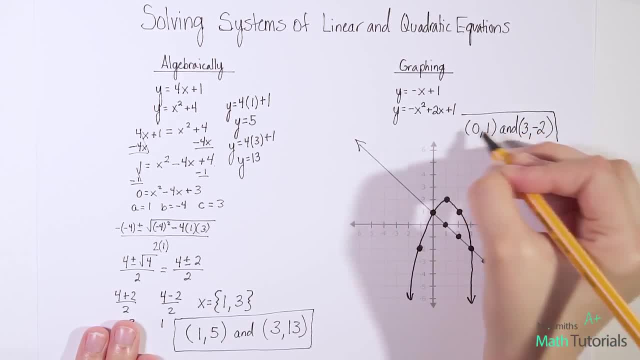 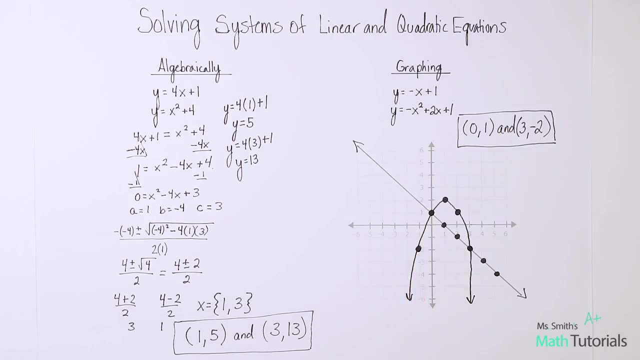 Okay, So those are my two intersecting points. Now it's important to note that these could intersect twice, Like we see here. Okay, Okay, So they could only intersect once. Like what if I had a line and it just barely touched one point and then it just kept going? 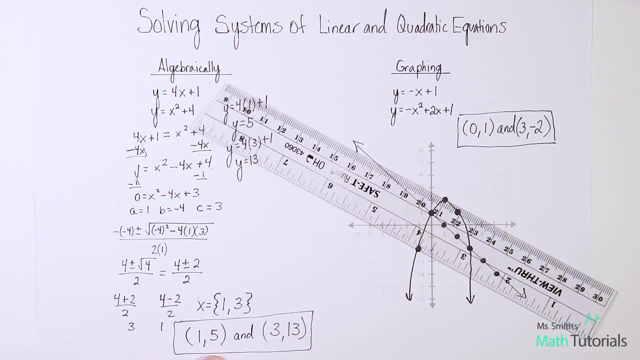 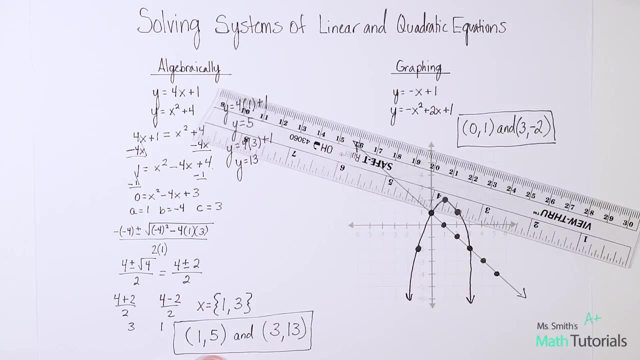 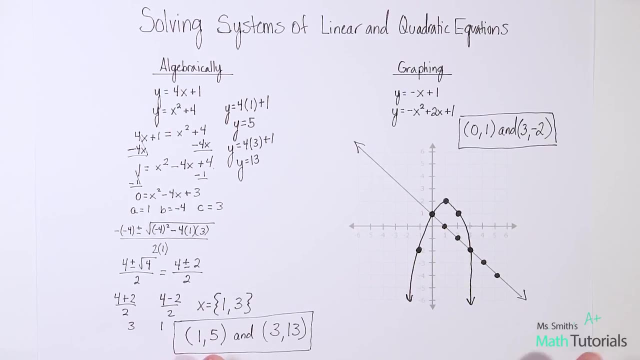 Okay, So that would be an example of if they only had one solution. or my linear line could be totally up here and not ever intersect that parabola And that would be no solution. So you can have lots of different types of answers within those three parameters. 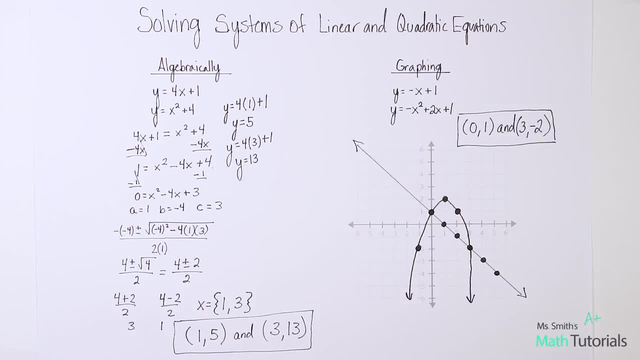 Okay, So you can have one solution, no solution, or two solutions. Those are your. those are your three options. Okay, Now just a trick to quickly do this on the calculator, I showed you the longest way, the second longest way, and now I'm going to show you the shortest. 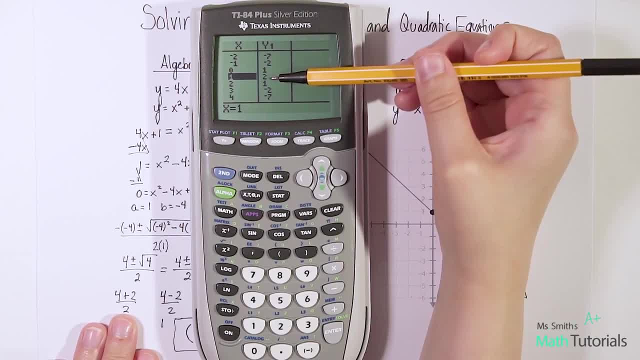 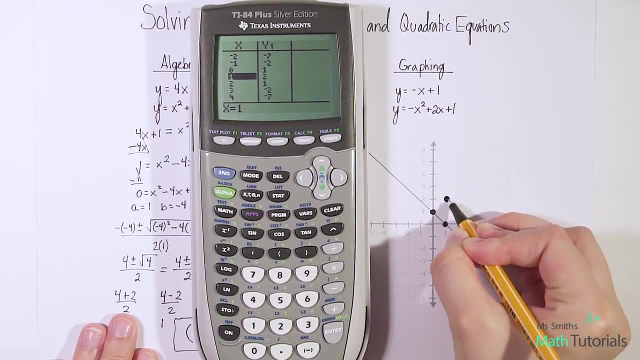 So it creates this kind of cool pattern effect. So you want to definitely have the vertex in there, which falls at one two. let me go ahead and plot that one two and then we'll plot around it. So then I've got zero positive one, zero positive one right there and negative one negative. 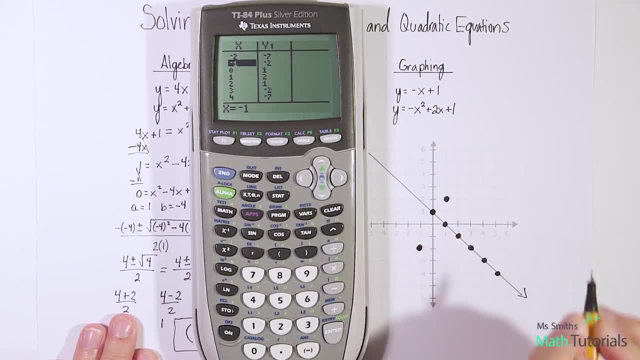 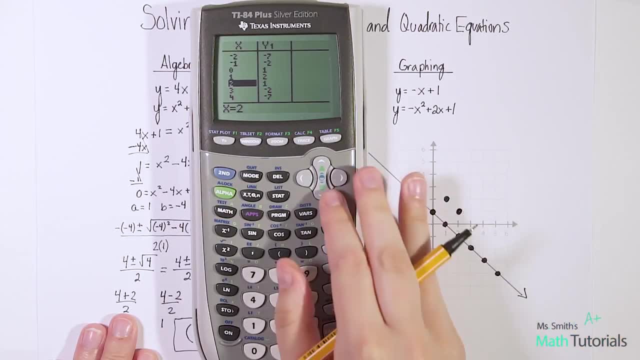 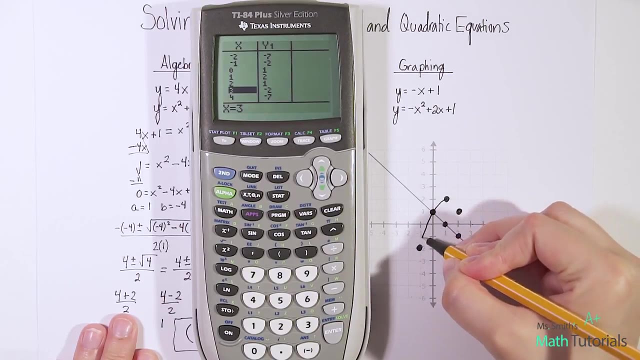 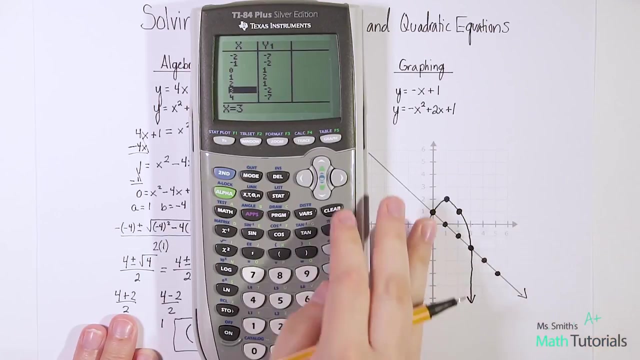 two negative, one negative two. Okay, Okay, Okay. So now I've got a little bit above the vertex. two, one, three negative two, all right, And we'll connect those dots in our parabola form. 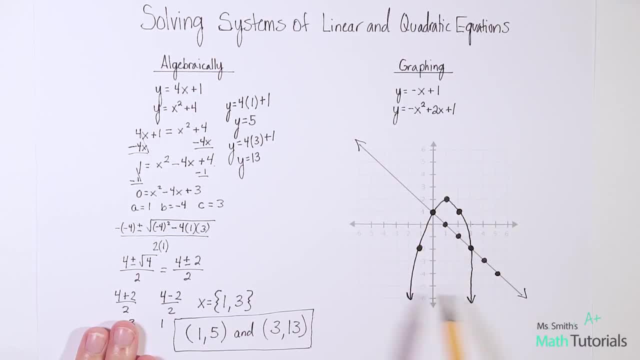 We want to physically see where. I've got my linear equation, I've got my quadratic equation. Where do they intersect? Well, I can. I can clearly see that they intersect right here at zero one and they intersect right here at three negative two. 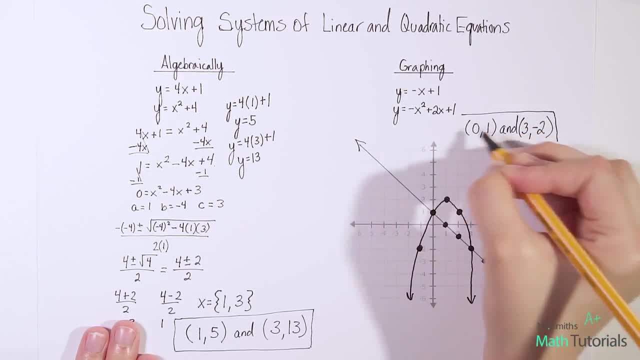 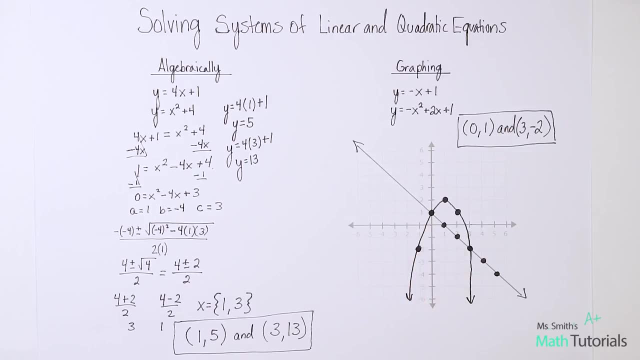 Okay, So those are my two intersecting points. Now it's important to note that these could intersect twice, Like we see here. Okay, Okay. So if they did only intersect once, like what if I had a line and it just barely touched? 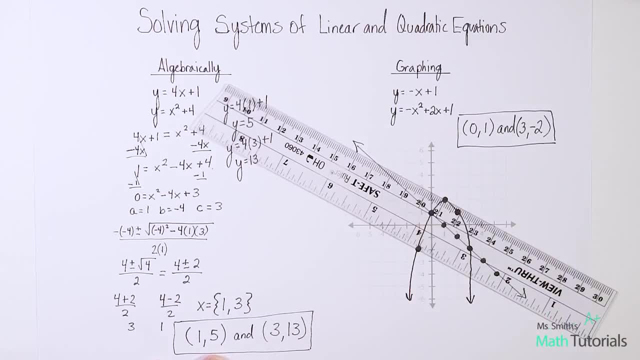 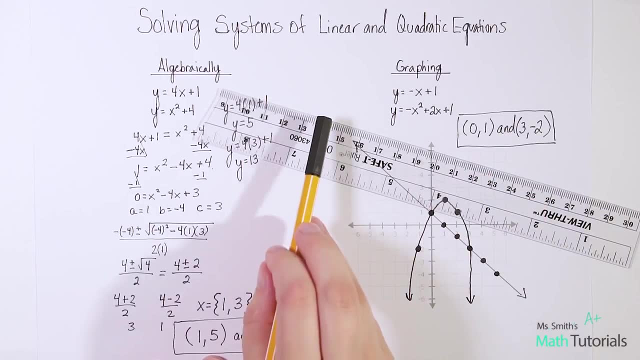 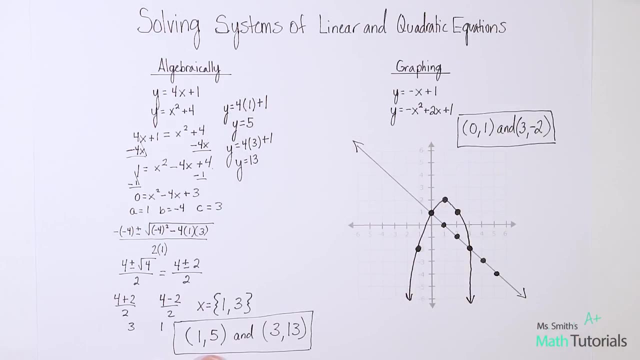 one point and then it just kept going. Okay, So that would be an example of if they only had one solution. or my linear line could be totally up here and not ever intersect that parabola And that would be no solution. So you can have lots of different types of answers within those three parameters. one: 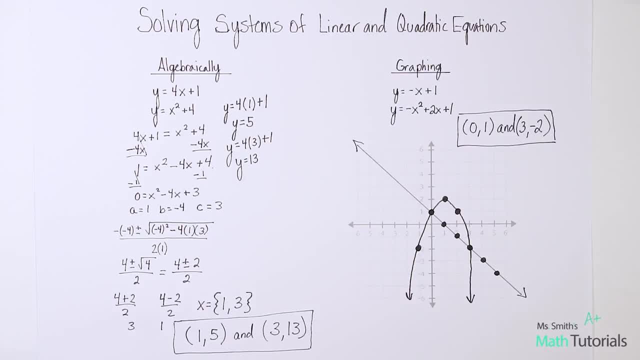 solution, no solution or two solutions. Those are your. those are your three options. Okay, Now just a trick to quickly do this on the calculator, I showed you the longest way, the second longest way, and now I'm going to show you the shortest. 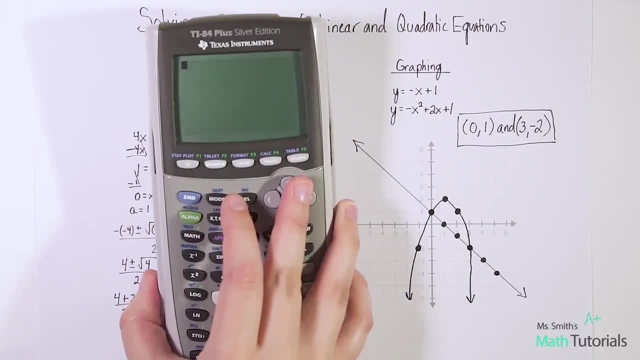 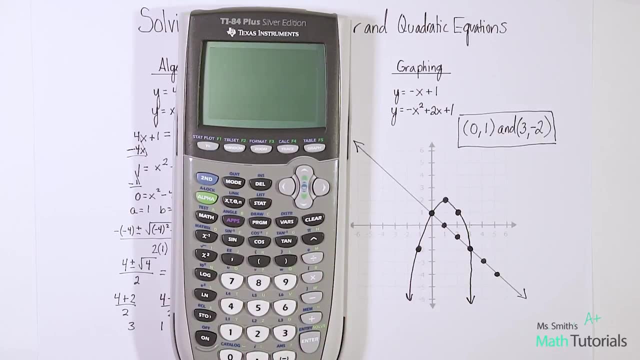 way. Okay. So assuming you do have a graphing calculator, first thing you want to do is clear it. So I've got a bunch of stuff in here from before. second plus seven, one, two, go ahead and clear it. I would want to go to my y equals and type in both of these two equations. 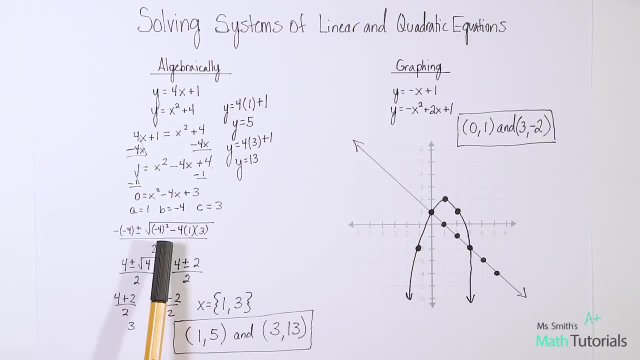 way Okay. So, assuming you do have a graphing calculator, first thing you want to do is clear it. So I've got a bunch of stuff in here from before. Second plus seven, one, two. Go ahead and clear it. I would want to go to my y equals and type in both of these two equations. Now, of course, I need to make sure that both of these equations are equal, So I'm going to go to my y equals and type in both of these two equations. 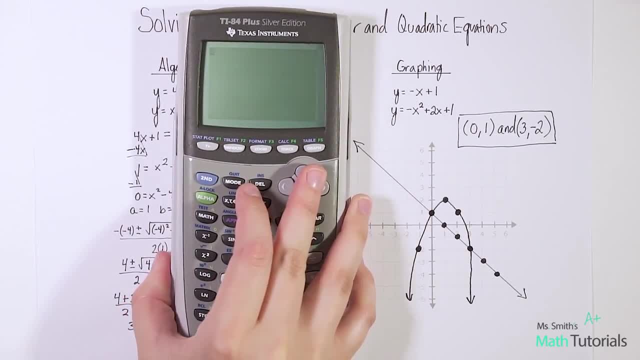 Now, of course, I need to make sure that both of these equations are equal. So I've got a bunch of stuff in here from before: Second plus seven, one, two. go ahead and clear it. Go ahead and clear it. 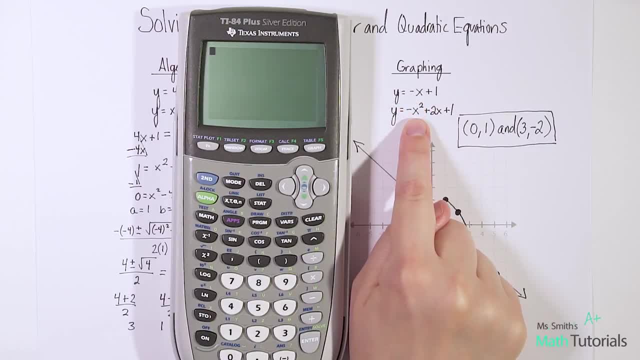 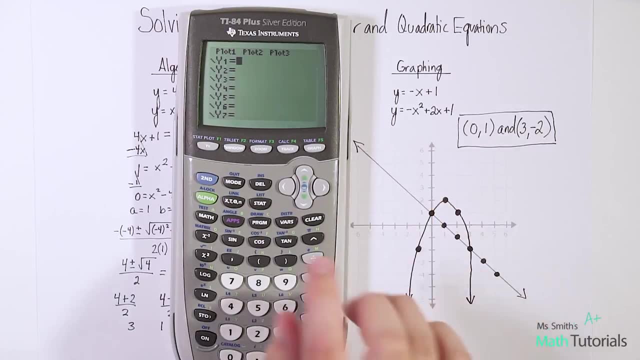 I would want to go to my y equals and type in both of these two equations. Now, of course, I need to make sure that both of them are set equal to y first, and they are, so I can go ahead and plug them in. 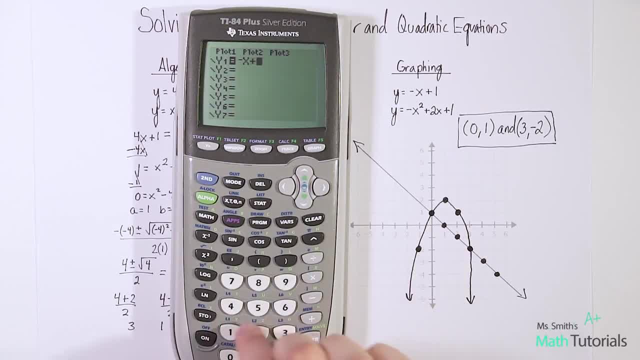 The first one says negative x plus one. The second one says negative x squared plus two, x squared plus 2x plus 1.. And my order doesn't matter here, right, I could have done this one first and that one second. It doesn't matter, Let's graph and let's look at these. Okay, there's my linear. 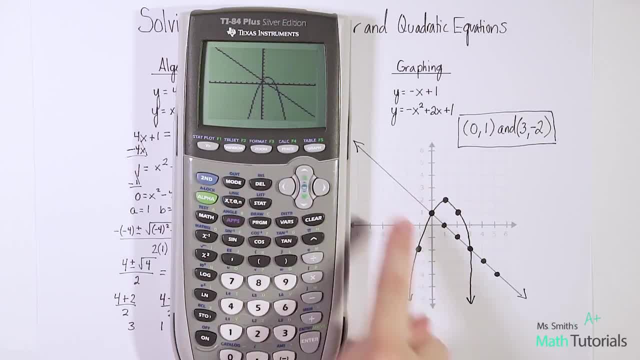 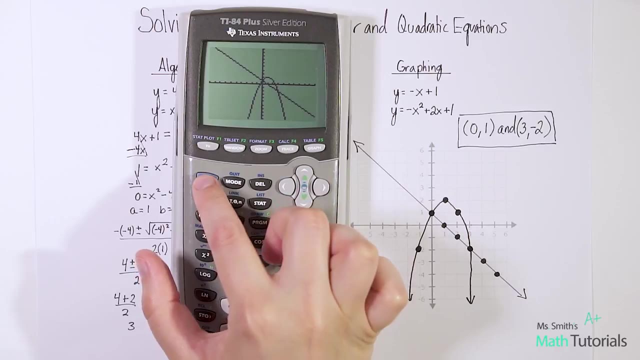 and there's my quadratic. And notice it looks just like what I graphed here, So we'd be able to get kind of like a shortcut to that picture. In order for me to find those intersecting points- because I would want to know what those points are- I just have to hit 2nd, trace 5.. And notice. 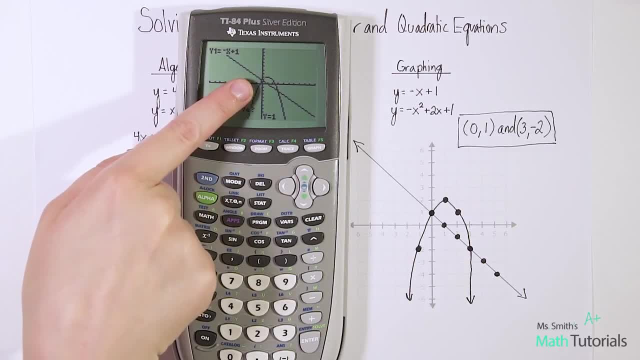 how one shows up right there. a little, I think of it as like a blinking spaceship shows up right on the intersection. All I have to do is hit enter three times: 1,, 2,, 3.. And it's going to tell me: 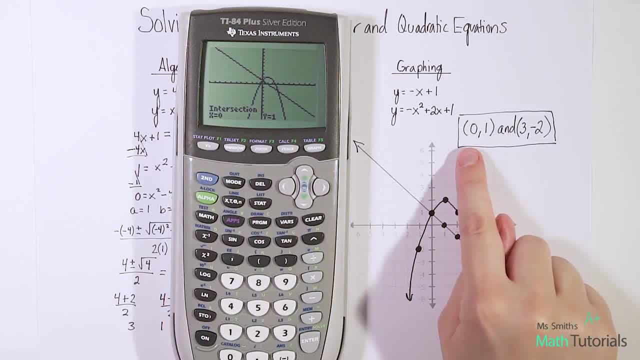 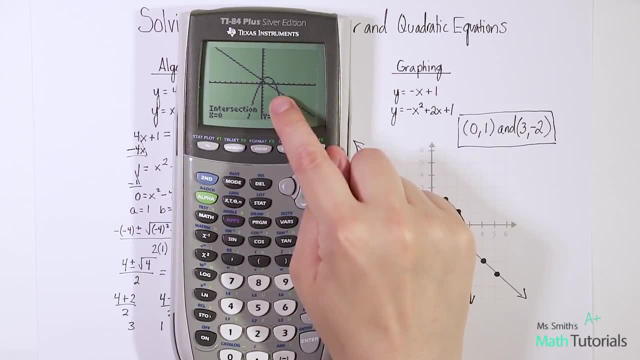 the intersection is at 0 and 1.. And isn't that what I got, 0 and 1.. But now I want to know the other intersection, Because there are two. I can clearly see two here, So I just do it again. I go 2nd, trace 5.. 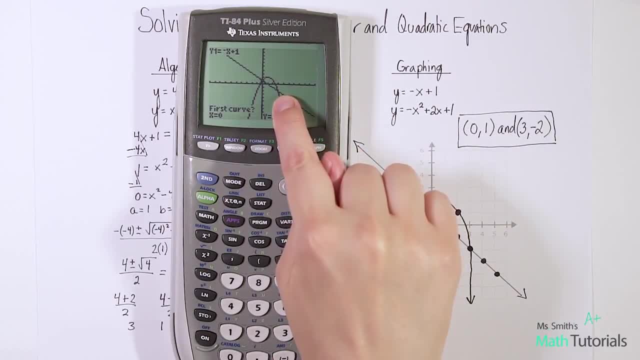 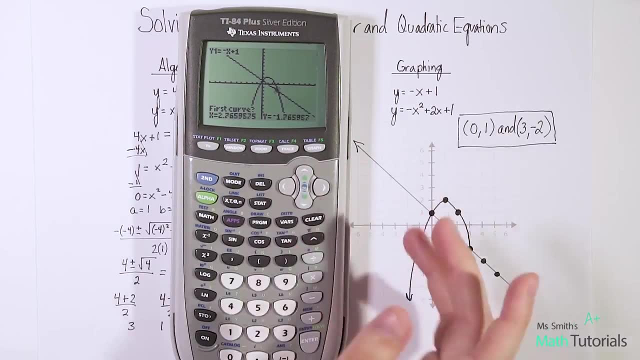 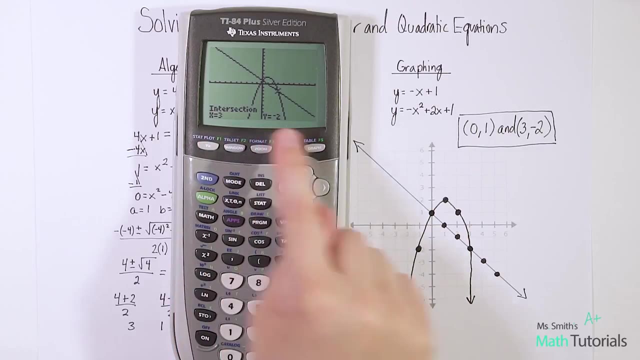 This time I'm going to take my spaceship over to the other intersection Right there And just get as close as you can. 1,, 2,, 3.. And see, I see my other intersection falls at 3, negative 2.. 3,. 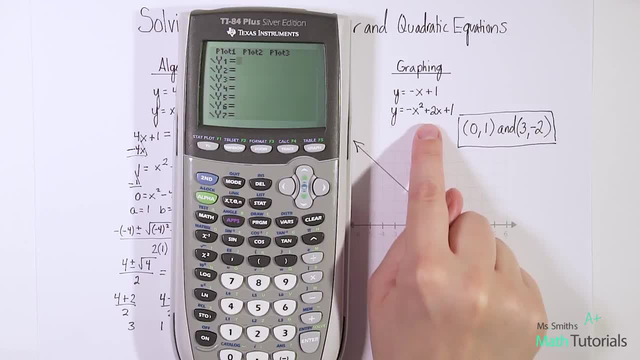 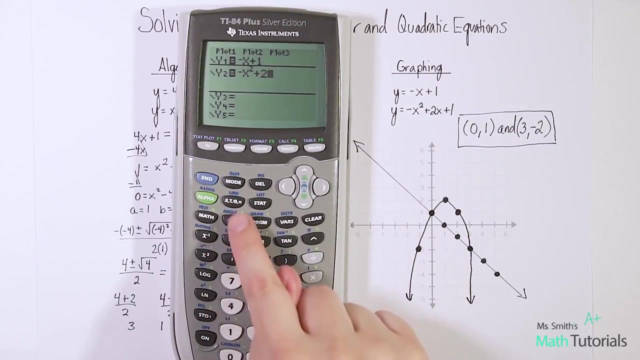 Now I want to make sure that they are both set equal to y first, and they are, so I can go ahead and plug them in. The first one says negative x plus one, The second one says negative x squared plus two, x plus one, and my order doesn't matter. 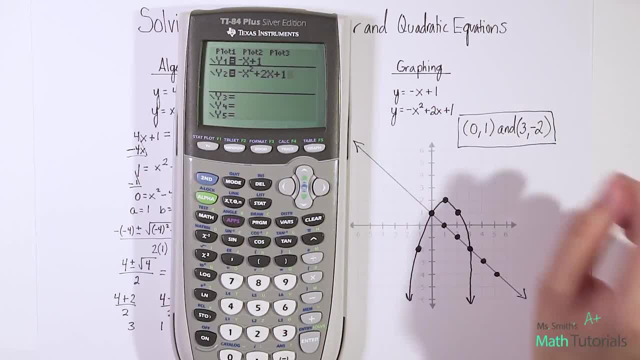 here. right, I could have done this one first and that one second, It doesn't matter. Let's graph and let's look at these. Okay, There's my linear And there's my quadratic. and notice it looks just like what I, what I graphed here. 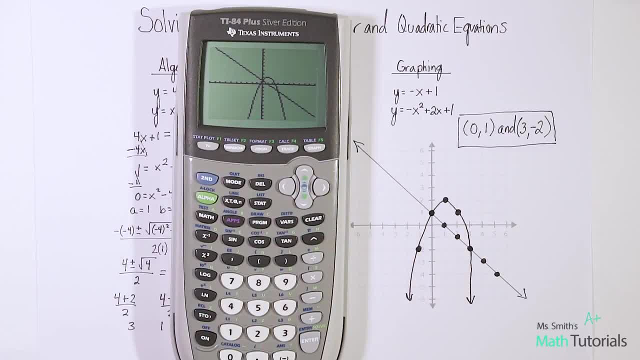 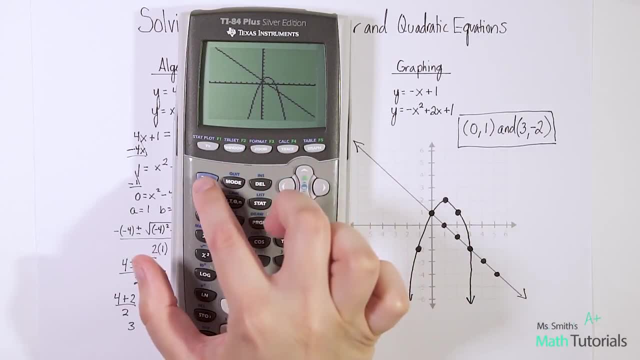 So we'd be able to get kind of like a shortcut to that picture. In order for me to find those intersecting points- cause I would want to know what those points are- I just have to hit second, trace five, and notice how one shows up right there. 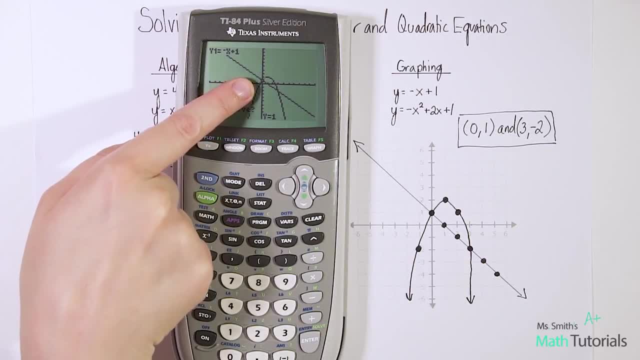 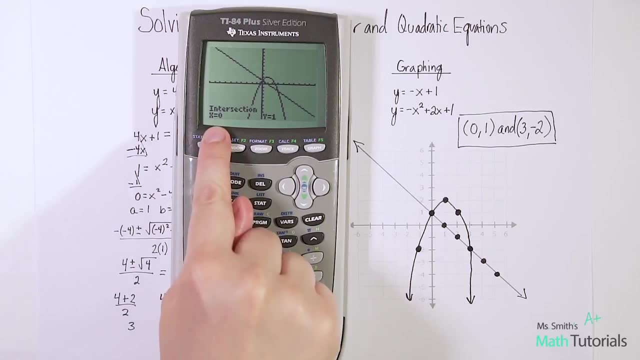 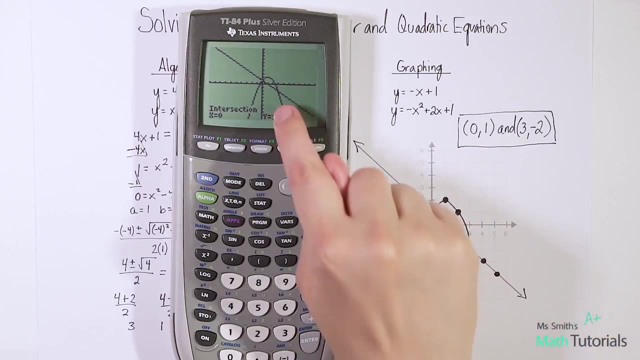 A little. I think of it as like a blinking spaceship shows up right on the intersection. All I have to do is hit enter three, One, two, three and it's going to tell me the intersection is at zero and one. And isn't that what I got: zero and one. but now I want to know the other intersection. 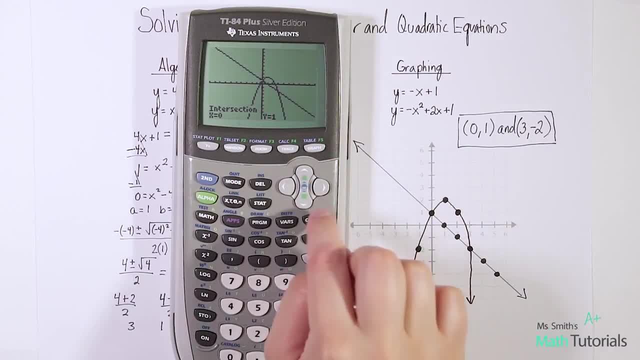 because there are two. I can clearly see two here. So I just do it again. I go second trace five. This time I'm going to take my spaceship over to the other intersection right there and just get it as close as you can. 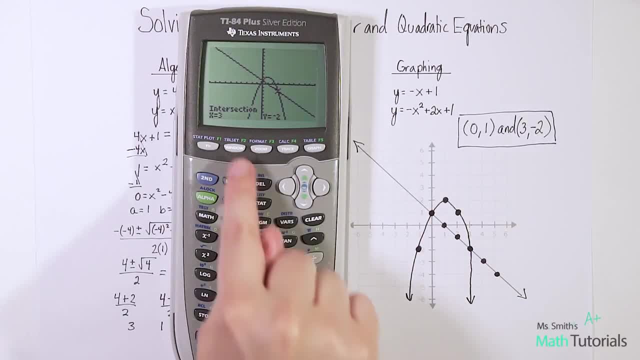 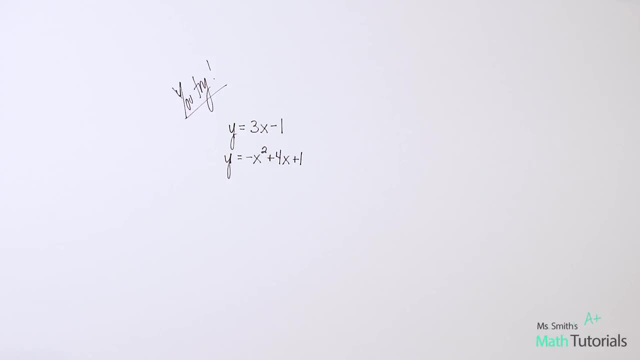 One, two, three. and see, I see my other intersection falls at three negative two, three negative two. Here's one for you guys to try on your own. I've given you a linear equation- Y equals three, X minus one- and a quadratic equation. 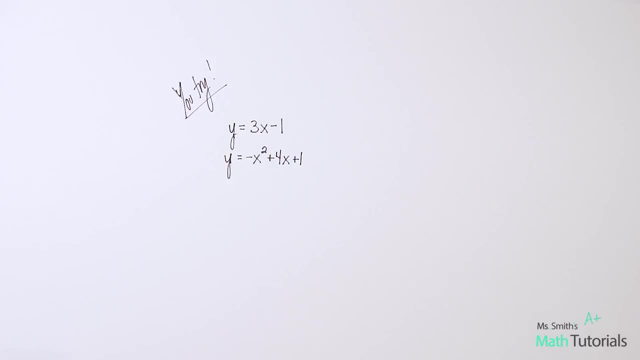